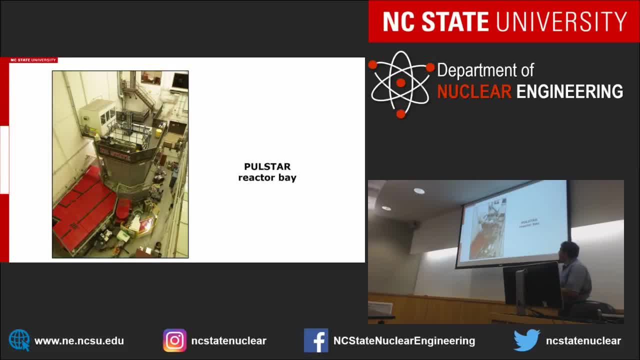 Polestar reactor is the first reactor and the main reactor I'm working with on a daily basis. This is our bay area And if you haven't visited this is something that you might want to do. take a tour and look at everything that we do. We have a very busy activity level in this reactor. 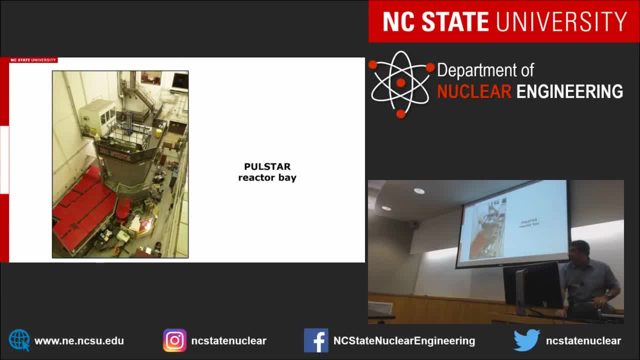 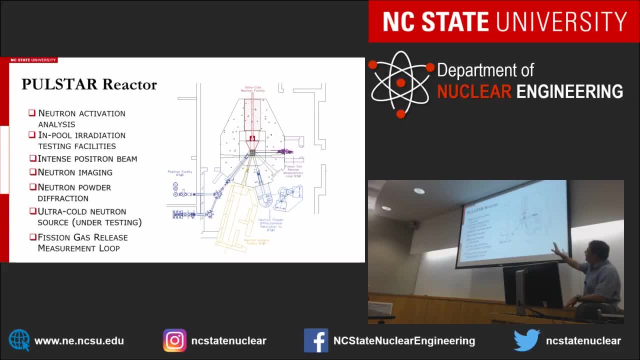 with all of the facilities that we have developed and all of the nature of activity. Just to give you an idea in a schematic fashion, we really view this reactor as a major radiation source and we're using the radiation emanating from the core of this reactor to design and set up. 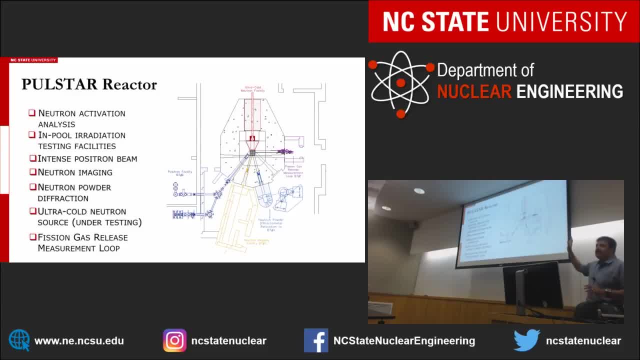 radiation probing facilities, including scattering instruments. using neutrons imaging instruments, We're using it also to generate positive ones, which are very important to us, And, if you want to build a Bhelium, to generate positrons and using them as radiation probes. 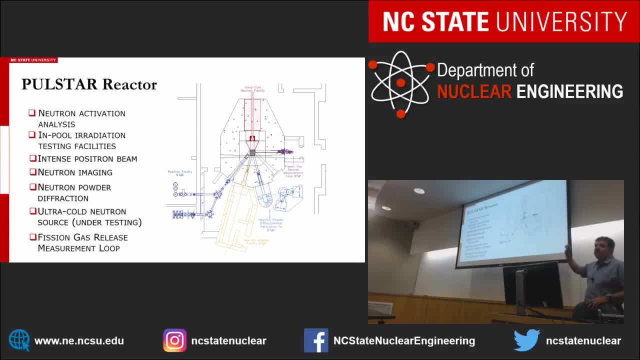 We have fundamental experiments going on with neutron physics and the use of ultracold neutrons. We have nuclear energy oriented experiments, where we are testing and building, and soon to be operating, a fuel testing loop here in the reactor. as you see, And this is going to be one of our main- 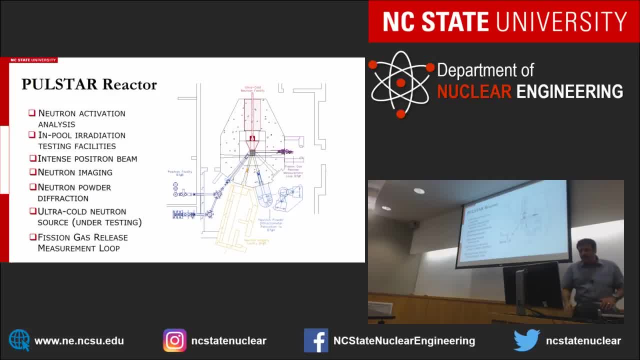 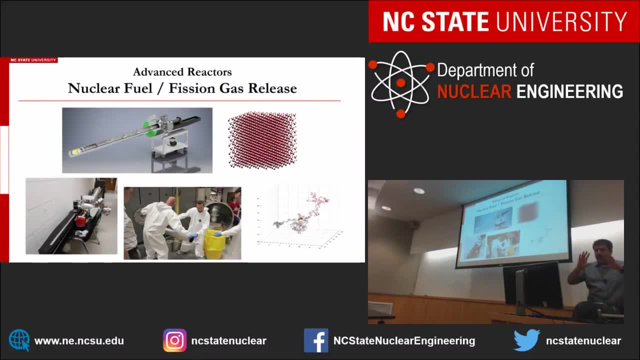 and newest facilities going online in the very near future. But in addition to doing all this and all of the work that we do, that I thought of the theme that our group is really moving into And we really move in a theme that you could consider. 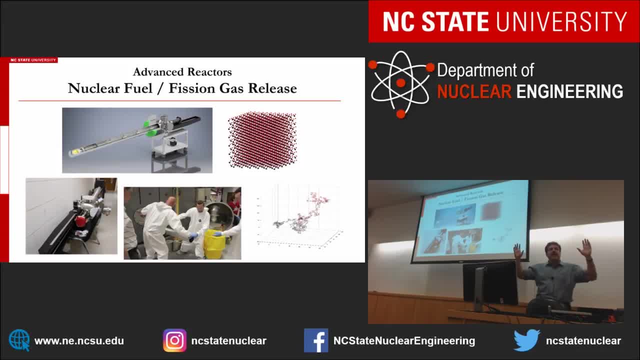 as a general umbrella for the title of Advanced Reactors, Because everything that we do in terms of the fuel research, in terms of the fundamental physics analysis, that we do in terms of the development of instrumentation and detection techniques, All really falls, whether programmatically. 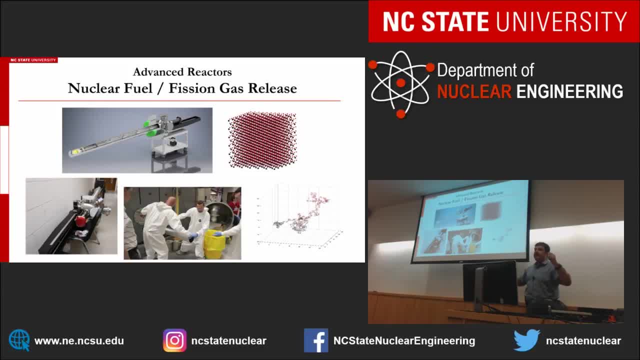 from a funding point of view, or even scientifically and engineering wise, under the Advanced Reactor umbrella. And this is the loop, And I put it here on purpose. This is the loop that we are designing, And some people may recognize these figures. I think is it you, Cole, that made this. 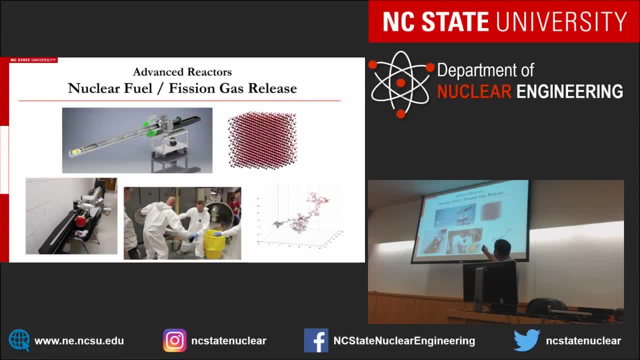 OK, So I'm guessing right, Because I was wondering where these figures came from. And this is a schematic of the loop that we're building And we're actually testing its insertion. you can see here We're also looking at fundamentally what this loop is going to generate for us. 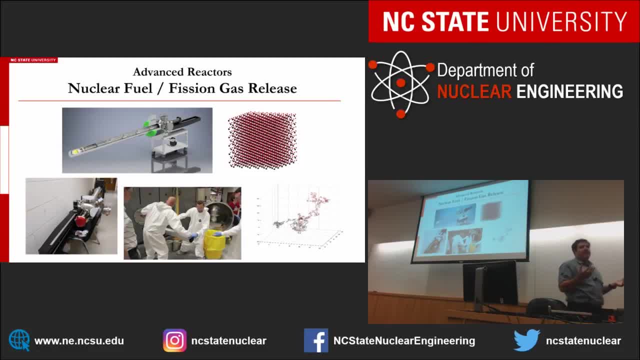 It's going to generate information about the release of fission gases from advanced nuclear fuels And we're trying to understand how this release happens on an atomistic scale. So we're resorting to atomistic simulation techniques to not actually model the atoms, but we're actually 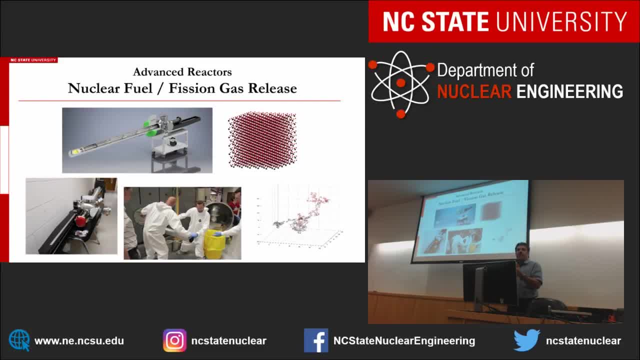 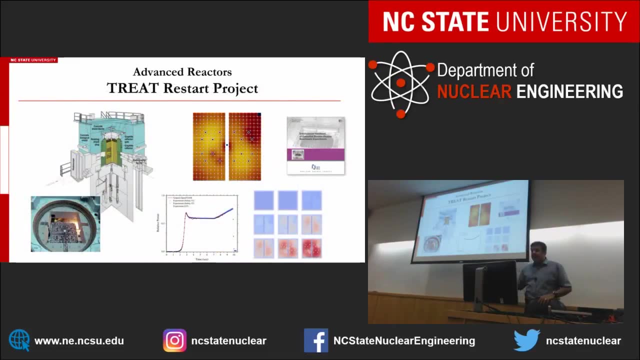 modeling the vacancies, almost like modeling the inverse Of matter, the lack of matter, and trying to track how these vacancies move around, because they are actually the main mechanism by which fission gases move in nuclear fuel. Another project related to this is: we are also 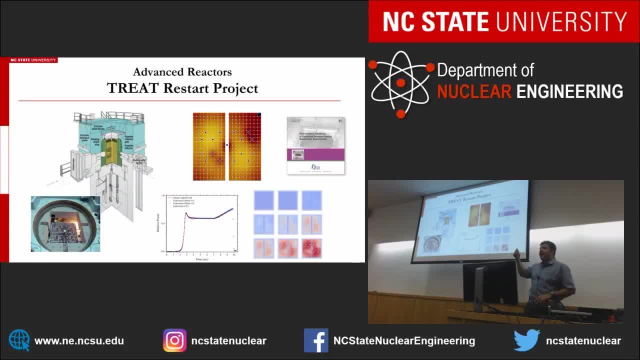 helping restart the treat reactor at Idaho National Lab and the testing of nuclear fuel, And Colby Sorrell here is working on that heavily And I think these are pictures from you right And what you could see here. this is treat Treat is a pulse. 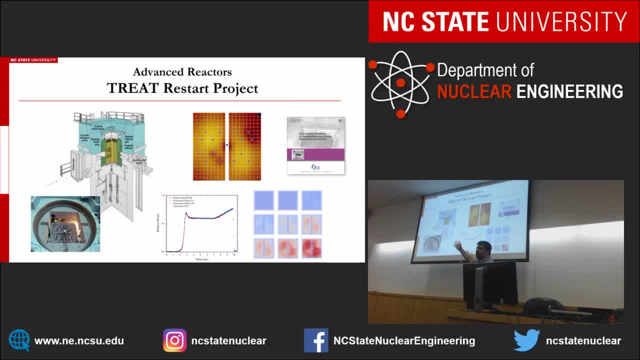 It's a pulse reactor that has just gotten restarted after about 25 years of hiatus. We are actually modeling the transient operating phenomena And I show here a transient with experimental and computational predictions of the transient and the evolution of energy distribution and temperature distribution. 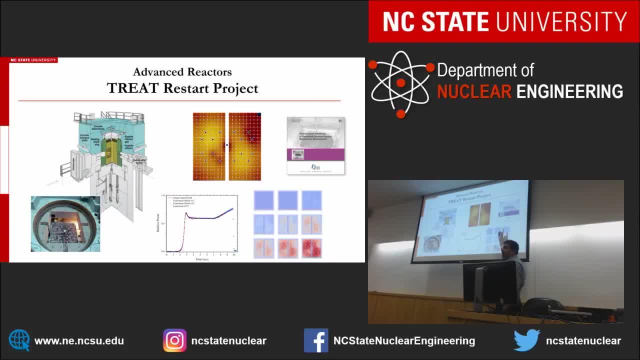 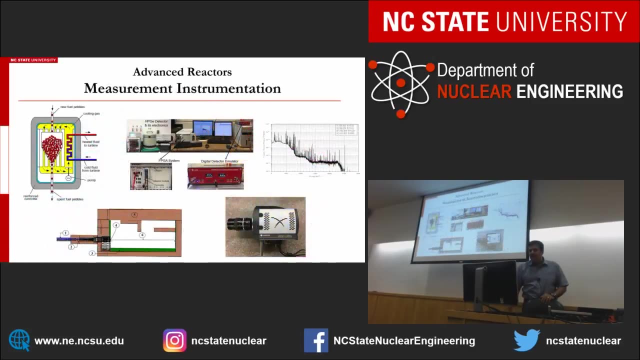 in the core And we're hoping to be able to contribute our transition, And we're also working on a whole series of simulations coupled to the experimental data, to the International Reactor Physics Handbook, which puts together all of the international effort in benchmarking in a place that users can resort to. Again to support understanding fuel phenomena. we're developing very advanced instrumentation. By the way, this is a gamma spectrum, Just because there were questions about it. We're developing very advanced gamma spectroscopy and the other one is a very advanced one. 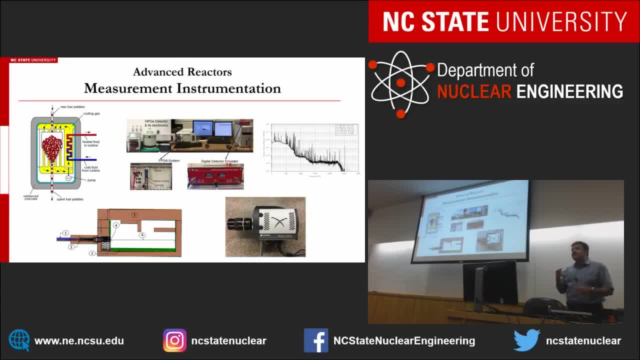 instrumentation. why is it advanced? because traditionally right now, when you go and you buy off-the-shelf gamma spectroscopy or spectrometry instrumentation, it's almost a one-size-fits-all. so you set it up and you leave it and it does the detection for you. here our gamma spectrometry: 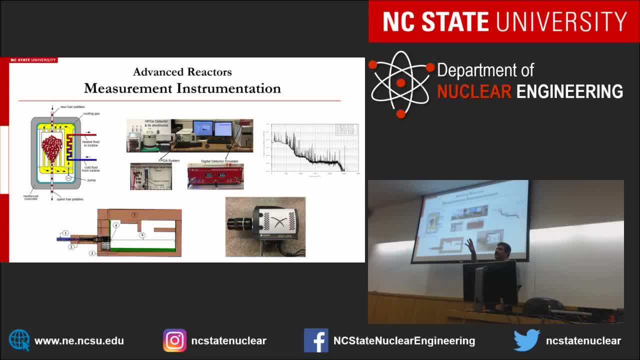 instruments actually look at the radiation environment and decide how they want to operate in that radiation environment. if the radiation environment is very hot and intense, the spectrometer will start adjusting itself to match that radiation environment and to collect the information in the most optimum fashion that results in the best resolution that. 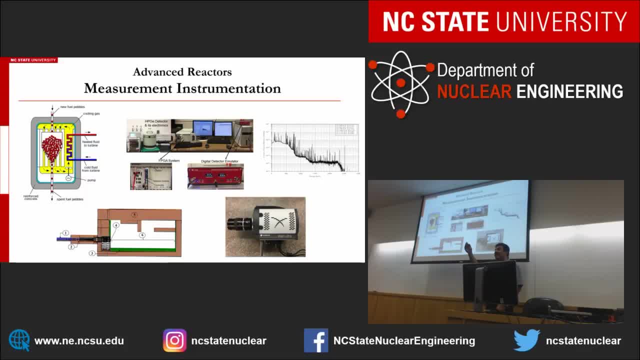 results in the best throughput and count rate without with the least loss of information. we're using FPGA technology to do that. we- some folks, I think, might be here who are dabbling with FPGA. you guys are dabbling with FPGA- is Shefali Saxon has been working on this for a few years now and she is near. 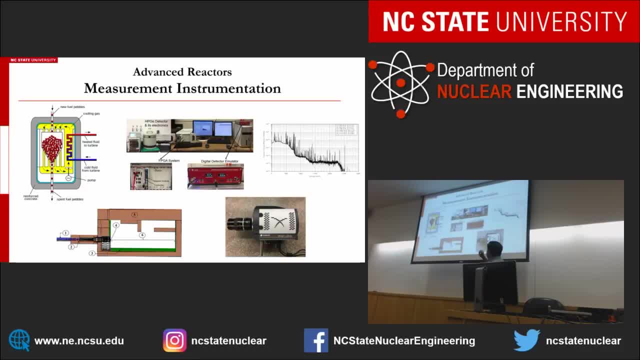 graduation with her PhD on this. we're also working on the visualization process, so we do a lot of imaging and we've just started installing our dynamic imaging systems in the reactor. again, one of our interest is to be able to image fuel structures and look at the damage in these fuel structures, and also 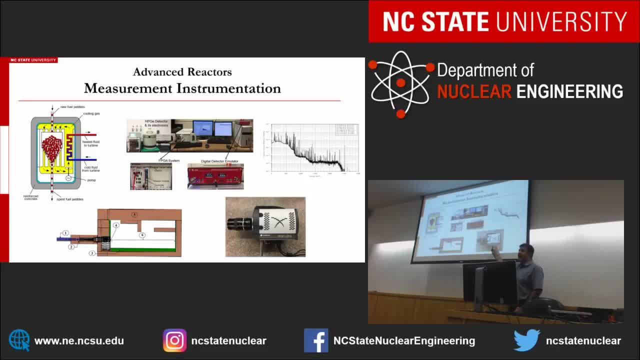 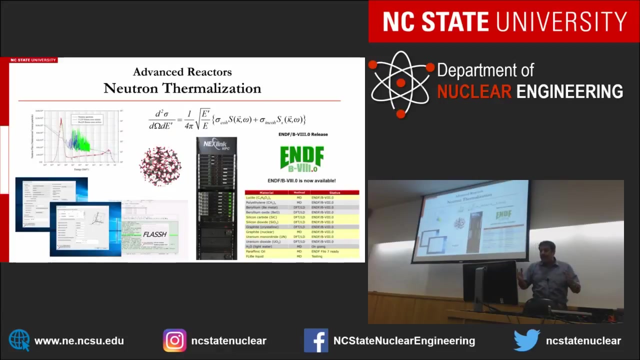 do it in a flow environment. so these dynamic cameras that we have been installing and using can capture flow environment, for example, and again, our thinking is that this would be quite applicable to advanced reactors like, for example, what would this be? pebble bed reactors- again advanced reactors- and neutron thermalization- this 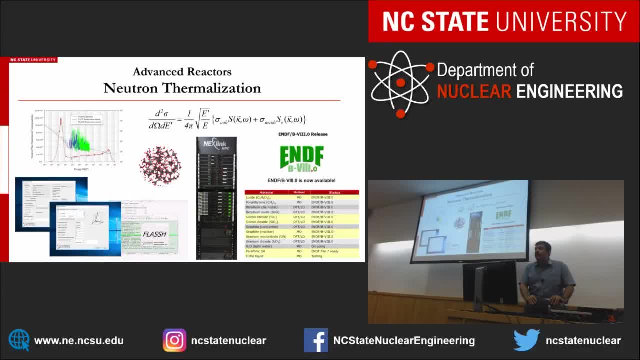 has been a staple of our operation and probably one of the biggest bill payers over here- and there are too many bill payers so- but this has been really a major piece of work that we started many, many years ago in this group and again, the motivation is to understand the operations of these reactors. you really 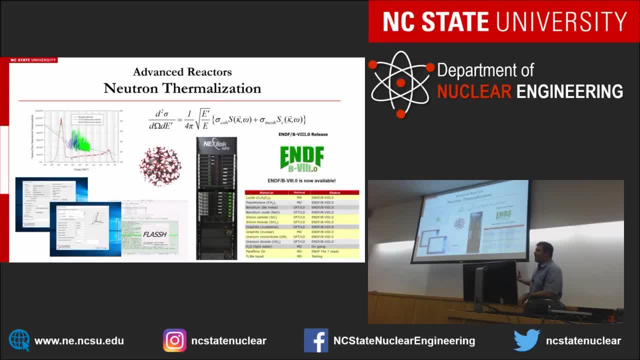 need to understand the reaction rates inside the reactor, and the reaction rates depend on the neutron spectrum in the reactor, and if you don't know the neutron spectrum accurately, everything gets thrown off, from basic operations to safety. one of the largest sources of uncertainty were the cross sections, especially at 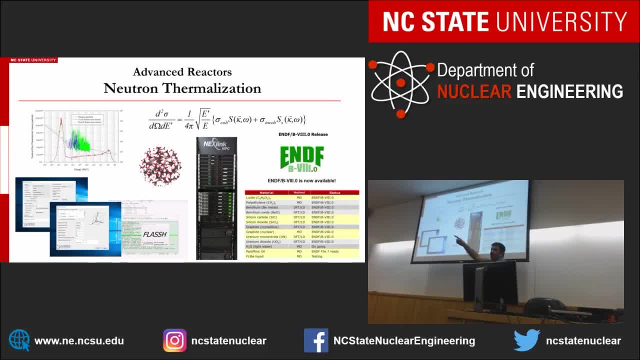 low energies. this is really the workhorse equation. my students over here have seen this too much. you can close your eyes if you don't look at it anymore and many of our group members right now are still working with a big contributor to the NDEF-8. so if you use NDEF data libraries and cross sections, 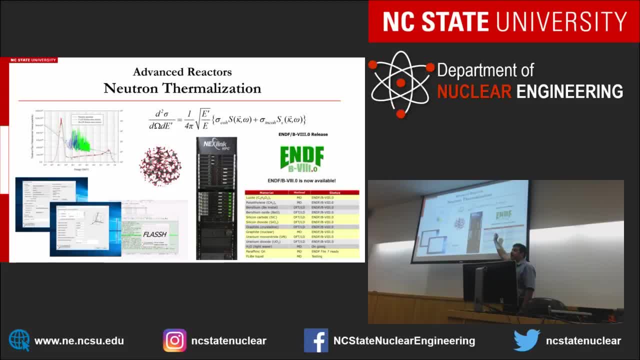 probably you are, even if you don't know it, if you're doing any kind of neutronics calculations, and these are all the libraries that we have contributed in the last two years, and so we have 11 libraries- I think there were 15- contributed to NDEF-8: 11. 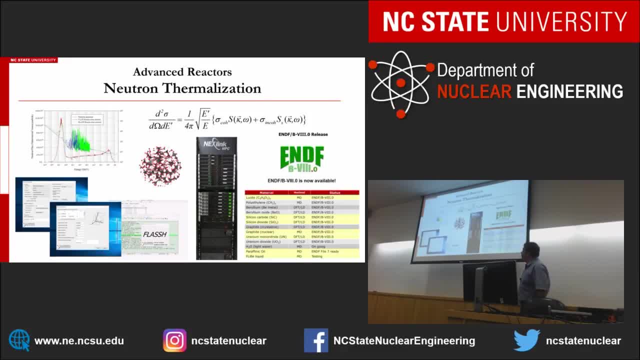 came from us at NC State, and so we are probably the largest in the world. we developed a new platform. we're aspiring to the play. who knows the enjoy data code? anybody used it, everybody knows it with. we think we can replace it. we have flash, and flash is a new system that now certainly replaces everything in enjoy. 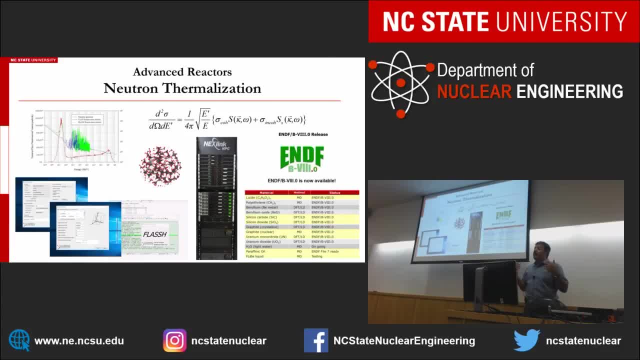 that deals with thermal scattering. we think that we can take it a step further and couple it to even higher energy treatments of the cross-section and if we do a little bit of work on that we're starting to think that we can take out the whole enjoy thing. but I'm not telling Los Alamos that yet because the 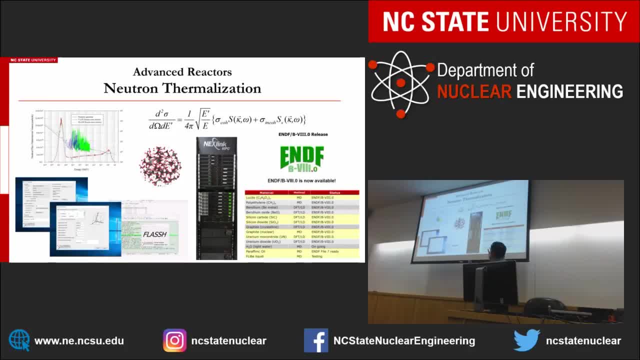 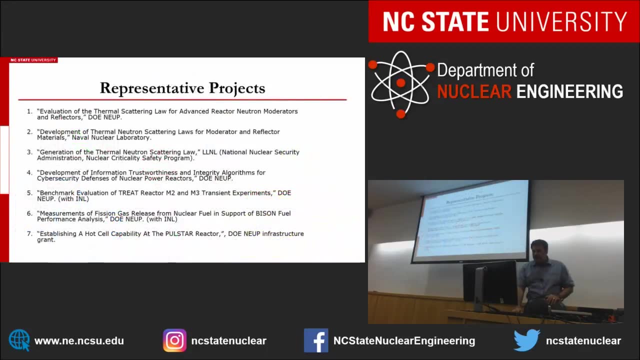 you know, I'm scared. I'm scared to say that. so we do a lot of atomistic simulations that support this, because really at the heart and soul, thermal scattering is sort of a area between materials and neutronics. it's a very special area, an interface area. these are representative projects that we have. we collaborate a lot with. 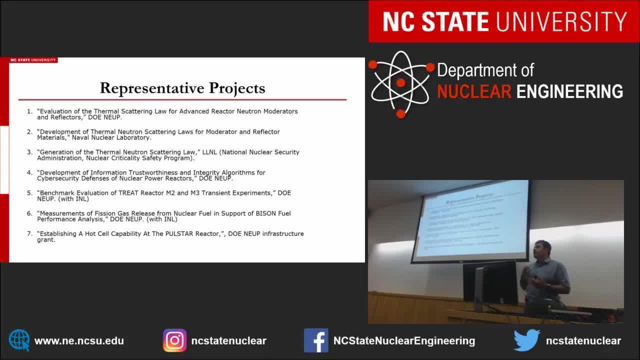 national labs and, of course, we're sponsored by government agencies like the Department of Energy, naval reactors and NSA, and so we have a lot of that going on. these are active projects. some of them are just brand new and starting, and we aspire to have more in the 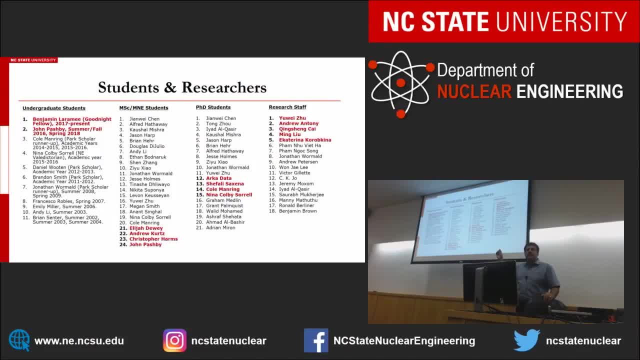 new near future. this is the family tree. this is the family for the past 20 years, so we have a lot of members in our family and the red ones are still at home and one day they will leave home. I know it's sad, but that will happen and